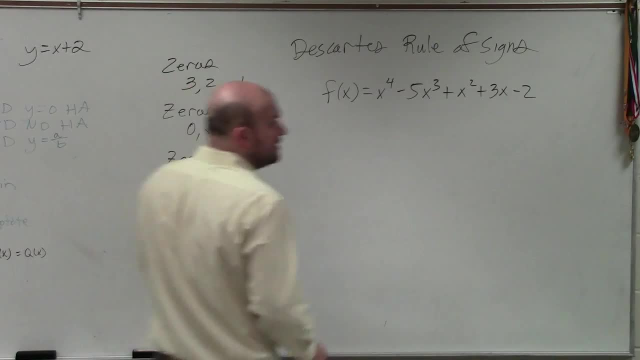 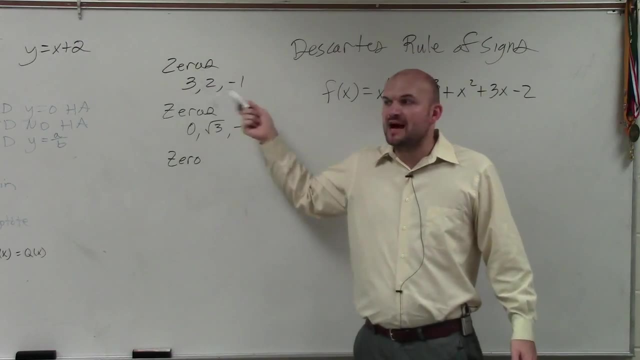 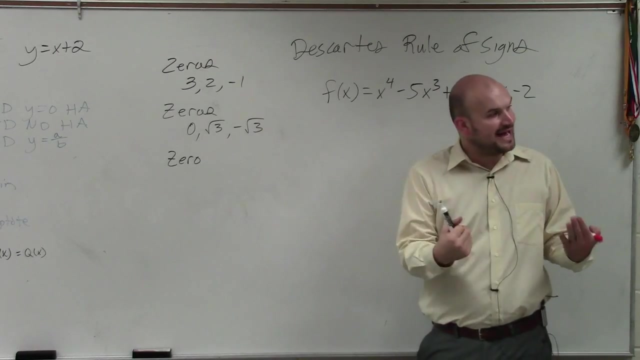 So so far we have found and we have found and we have written polynomials when given zeros that were rational numbers. We have found and written polynomials when we were given zeros that were irrational numbers. In the last homework we found and wrote polynomials when we had 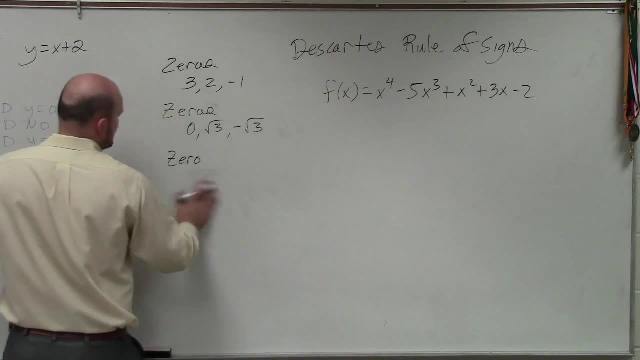 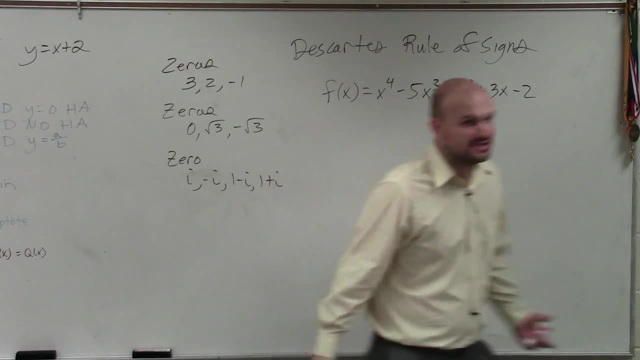 oh, let's just do this. i negative i, 1 minus i, 1 plus i. when we were given complex zeros, Correct, Right, We talked about i last class period. Yes, Anybody, Yes, Okay. 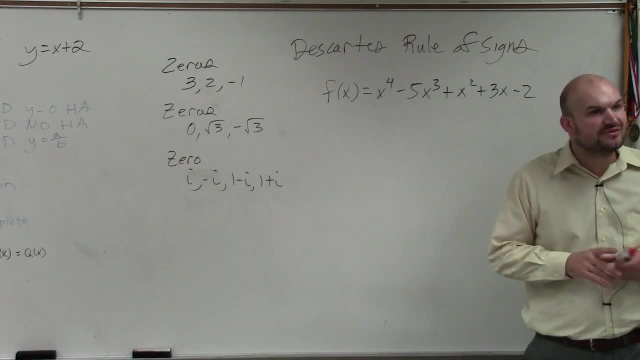 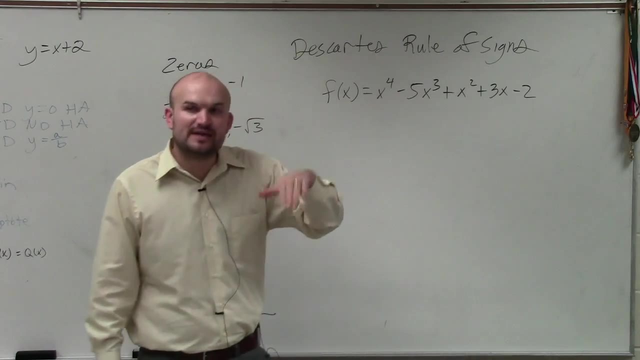 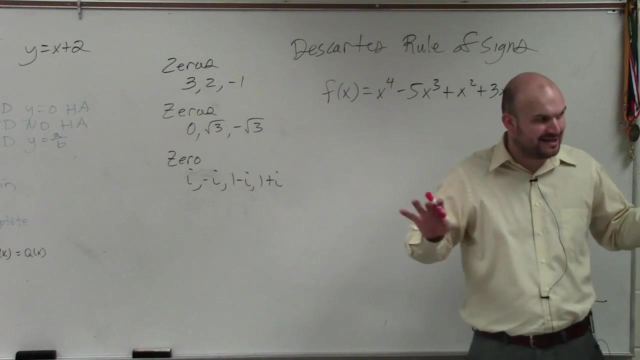 So what Descartes' rule of science says is based on the equations we can determine how many real positive and how many real negative, and therefore how many real positive and how many real negative. So we can determine how many complex zeros a function has without doing anything. 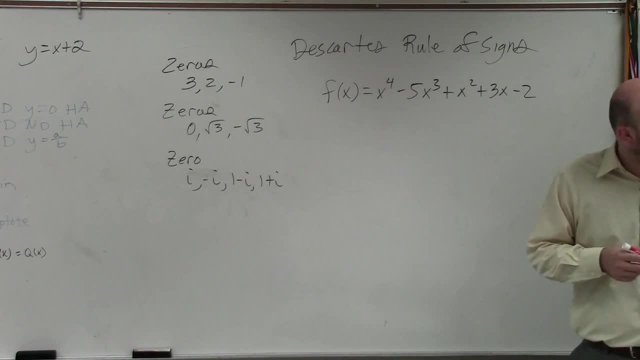 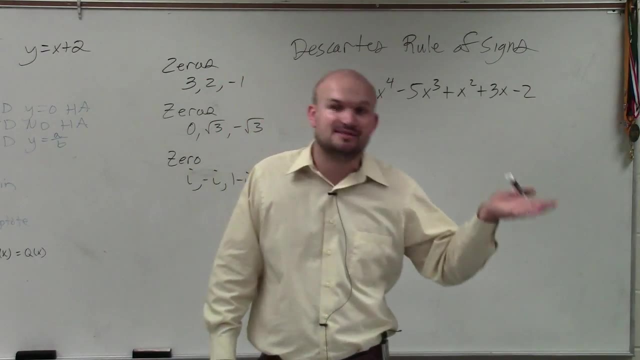 So well, it's just a way from inspection You guys can quickly. it's a good way to check your work And you might have a question that says: hey, to tell me how many complex, how many zeros and so forth. 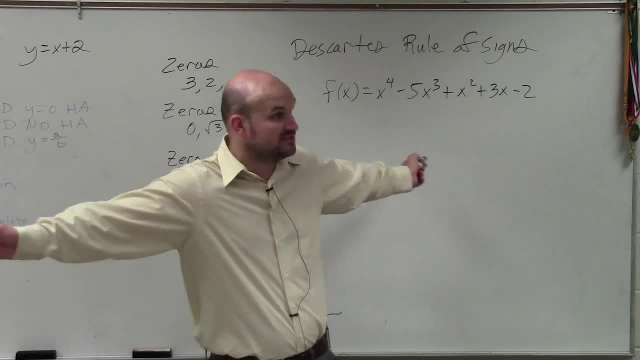 Well, without doing all the math that we've done- which you guys know, synthetic division sometimes can take a long time right, Without doing all the math, we can use Descartes' rule of science to answer that type of question like that. 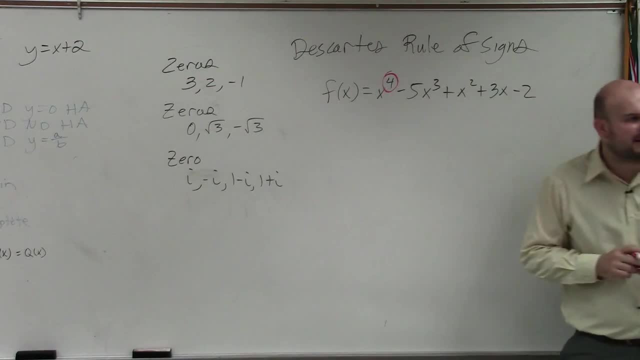 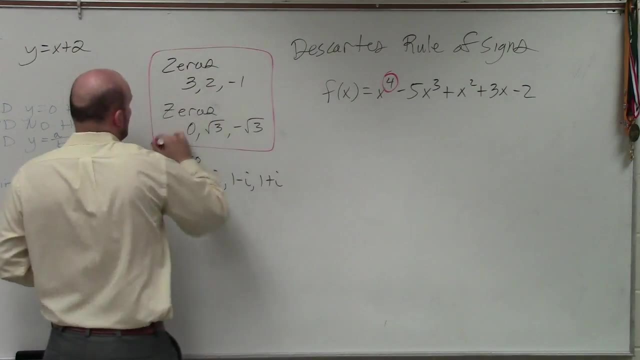 First of all, based on the degree, we know. how many zeros does this function have? Four, Four, Okay. Now, these are all real, Correct? Those are real numbers. You can plot those numbers on a number line, Correct? 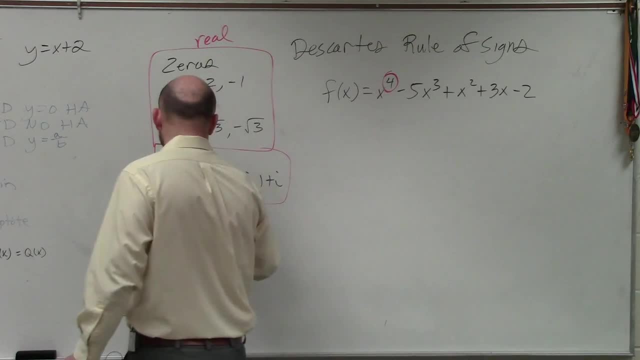 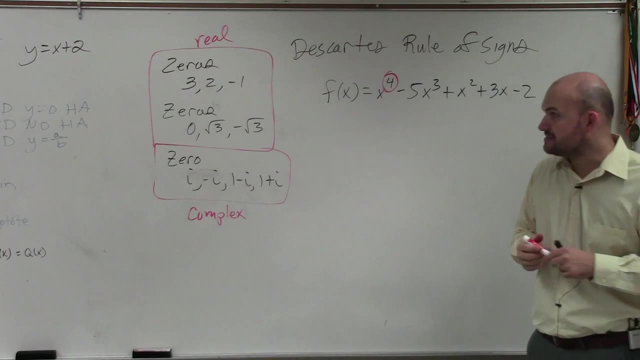 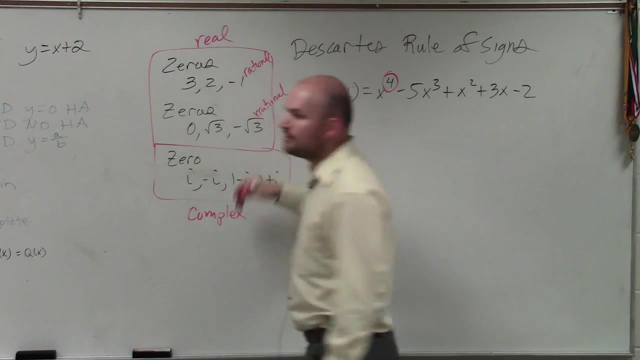 Correct. These are complex. You cannot plot them on a real number line. You can plot them on a complex number line, but not a real number line. Yes, These are rational numbers. These are irrational, But they're both real right. 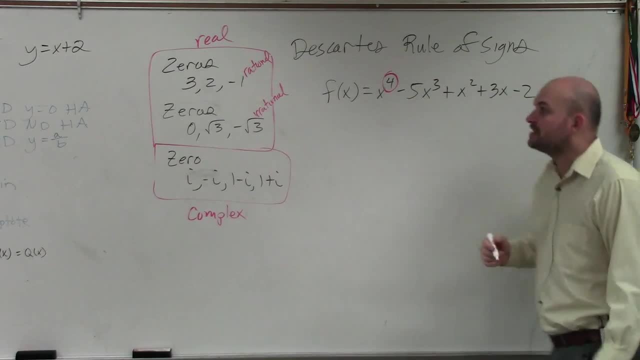 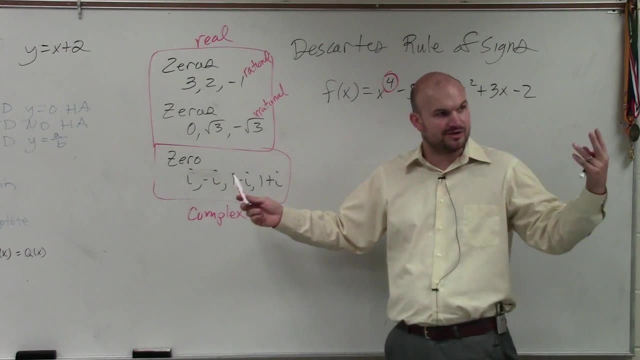 Some are negative, some are positive. okay, Also, just a note: remember zero. remember complex zeros always come in their conjugate right. They always come in pairs. okay. So what Descartes' rule of science says is: I can determine the number of real positive zeros. 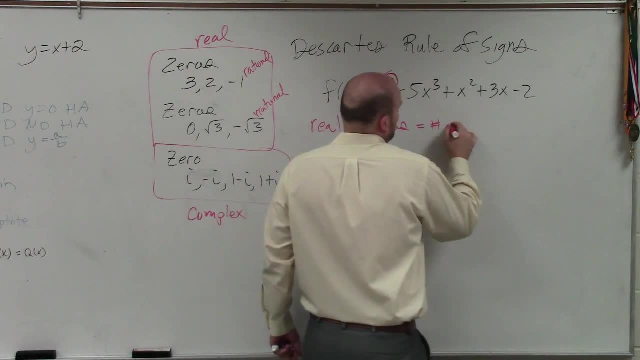 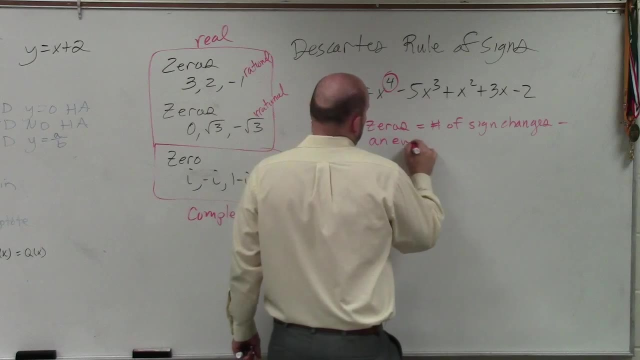 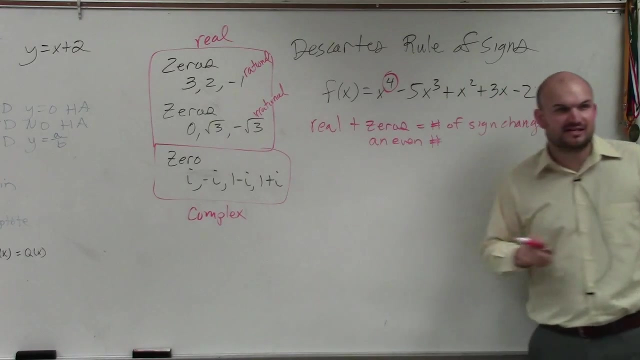 by the number of sign changes minus an even number, It kind of looks confusing. It's much easier just to do So. we start with positive x to the fourth, Then we go to negative x cubed. Do you guys see how I went from positive to negative? 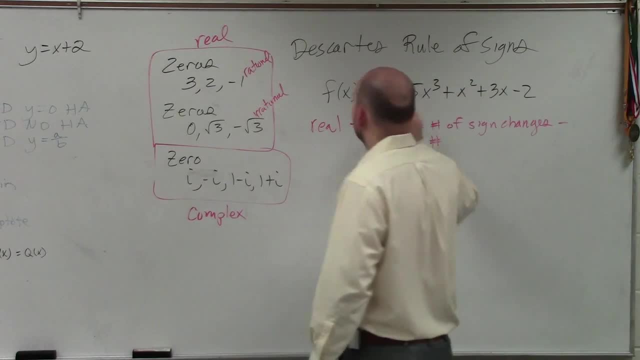 So I can have one positive real zero. Then I go from negative to positive, I can now have two, And then over here I have another positive change, Correct, So I have three real zeros, And then over here I have another positive change. 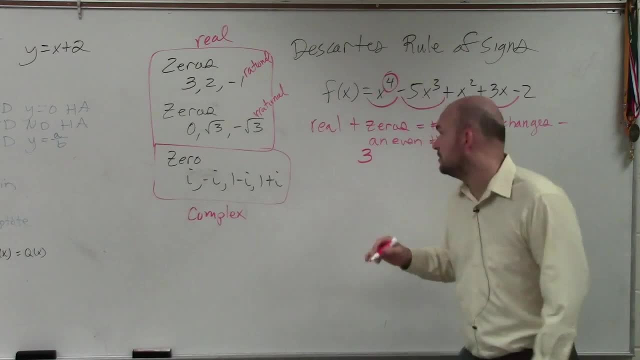 Correct. So I have three real zeros Or minus an even number, which an even number is two. I have two, I'm sorry one, I can't subtract any other. even I can't subtract two from one again. 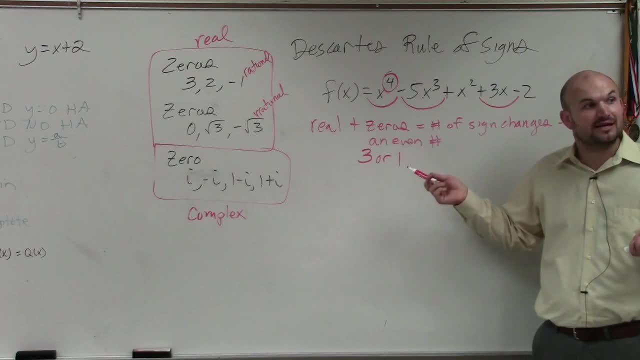 So I even have the option of three or one. Correct, Yes, Logan, I have a question: How does it matter what you subtract? Yeah, I mean, I can't subtract any larger number than two, But if you had like ten, 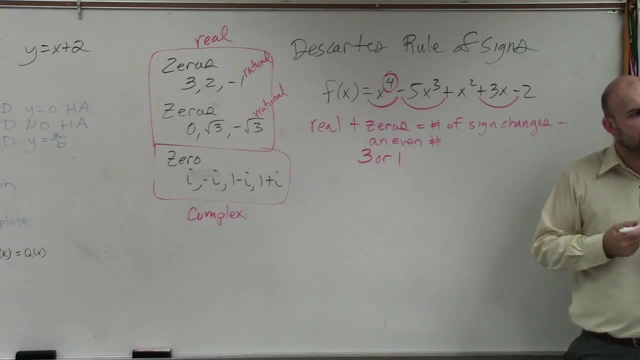 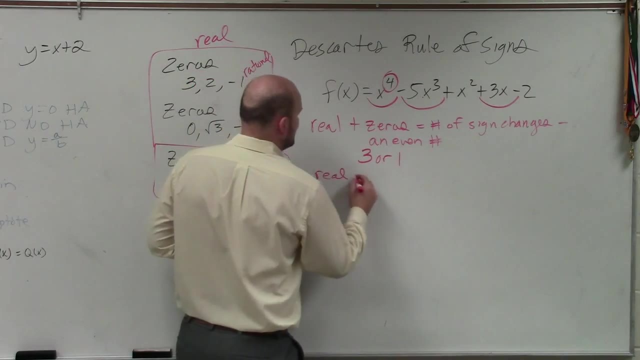 it would be ten, eight, six, four, two zero. Okay, what is that? Yeah, what would that be? I'm going to explain. I'm not done yet. That's the real positive. What about the real negative zeros? 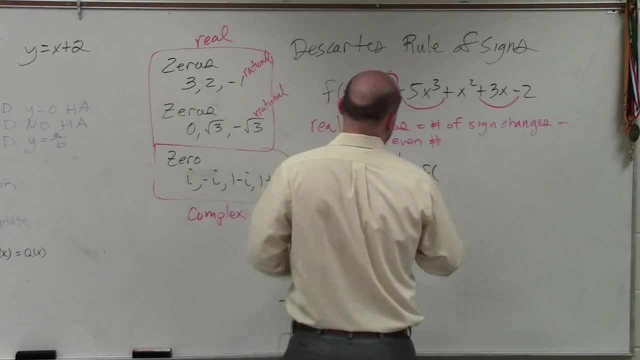 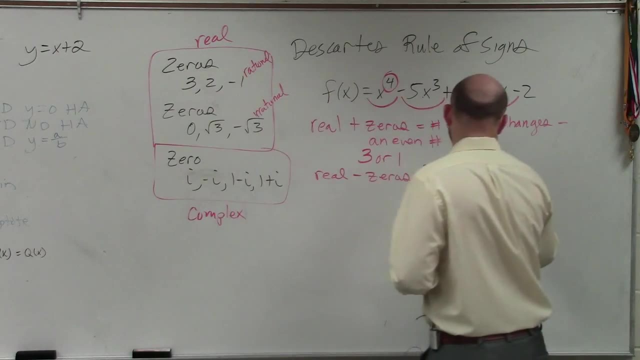 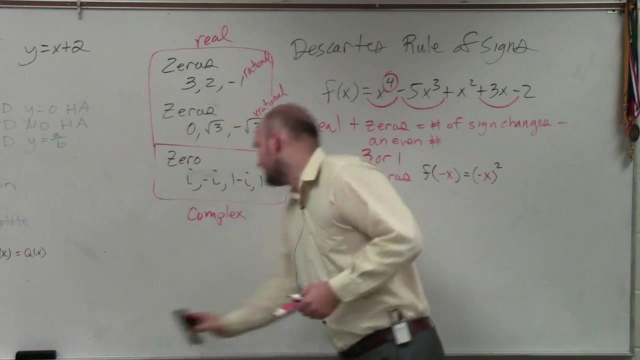 It's the same thing, but now we need to evaluate for f of negative x. So now we're going to plug in f of negative x. You guys, I think, want me to plug that in, So Actually I don't got time. 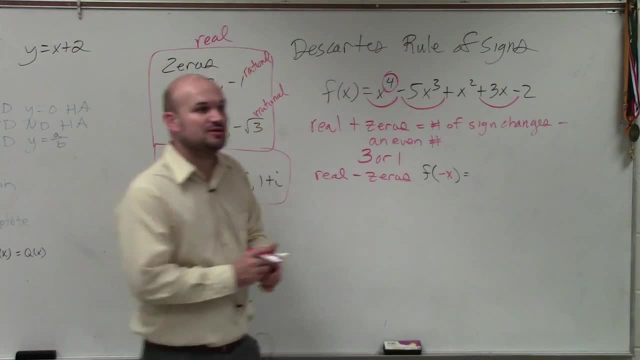 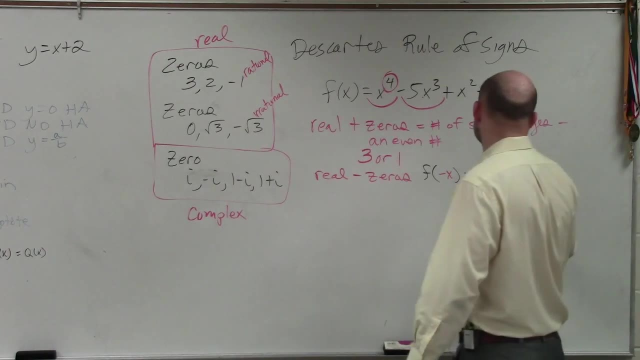 I got to move on. So negative x to the fourth is just going to give you a positive x to the fourth. Negative x cubed is a negative x cubed times. negative five is going to be a positive five x cubed. This gives me a positive. 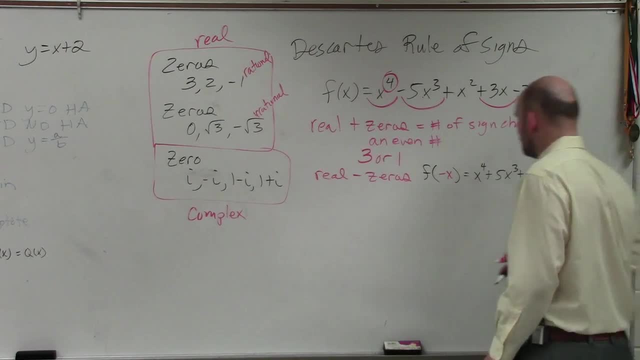 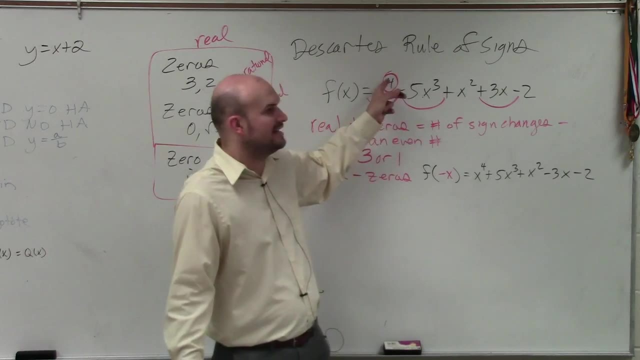 x squared minus three, x minus two. Does everybody see what I did? I just plugged in negative x and then simplified: Anytime you have a negative number raised to an even power, it becomes positive. Anytime you have a negative number raised to an even power.